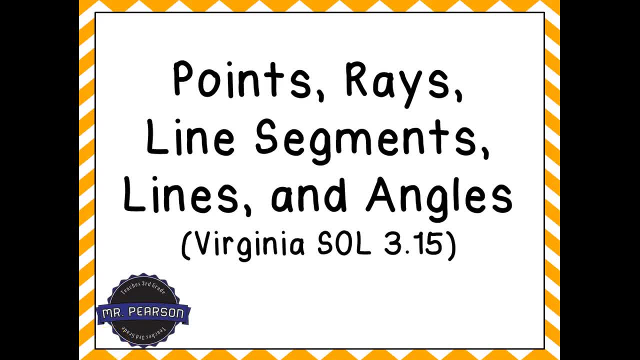 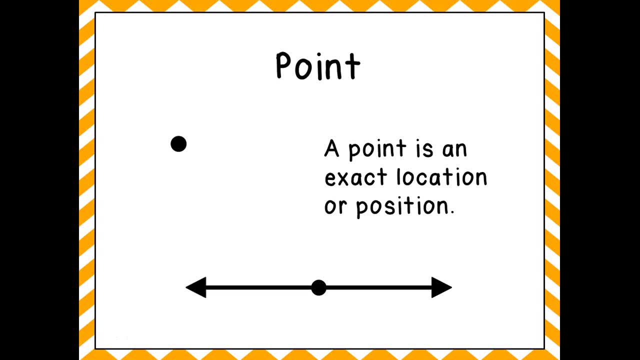 Points, rays, line segments, lines and angles Per Virginia, SOL 3.15.. Okay, let's take a look at these different shapes. The first one we have is a point. It looks exactly like this. It's just a. 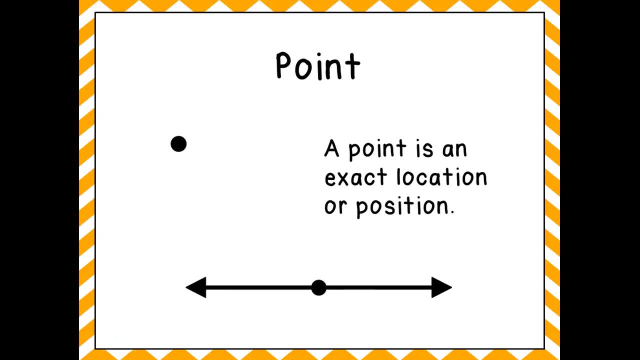 dot And a point is an exact location or position. You can see on this picture here. we have a point right there in the middle. So a point is just a dot, It's a space Exactly right there. All right, the next one we have is a line, And a line is straight and it continues in both directions. 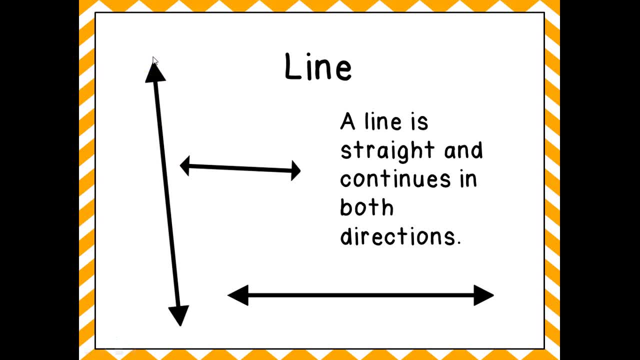 Take a look at this one right here. You see the arrow. it's pointing this way. It's telling me that that line is going to go on forever in that direction. Down here we have this arrow pointing downward, meaning the line continues moving in that direction as well. 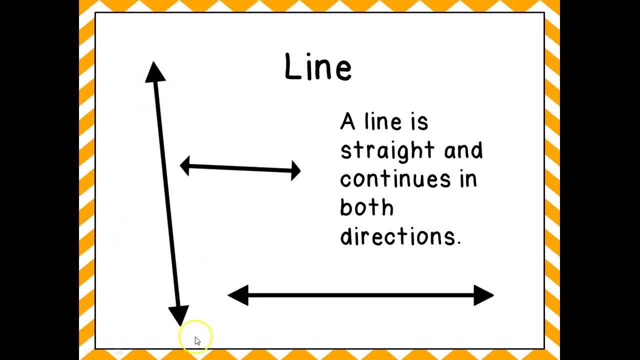 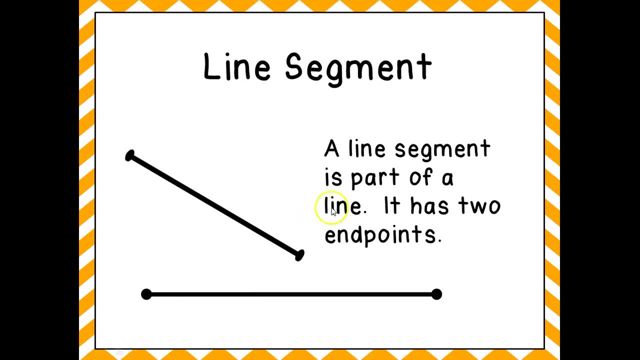 The way we can tell it's a line is because it has two arrows on either end and it's straight. Next, we have line segment, And a line segment is part of a line. So if you think about the line we just looked at, that goes on and on in both directions. a line segment is just a small piece. 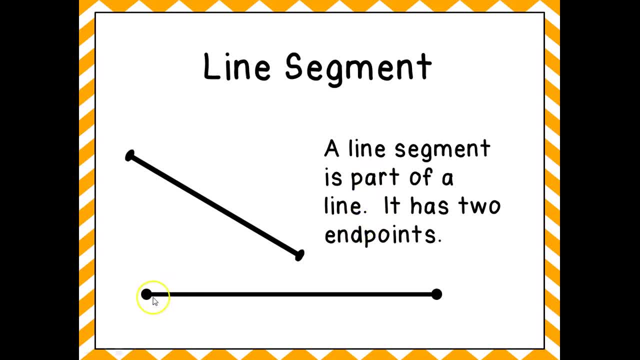 of that line And it has two end points. You see, here here's one end point. That's where it begins, And here's the second end point. Over here is where it stops. It's just a piece of that line. 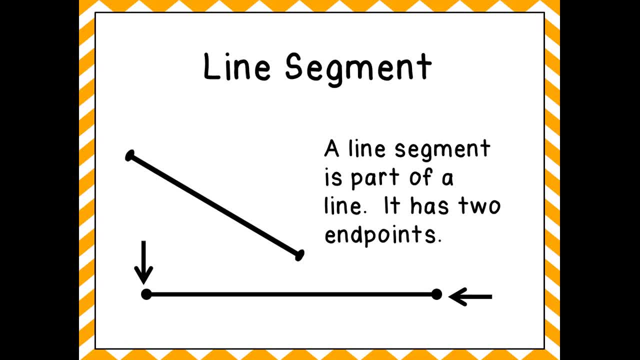 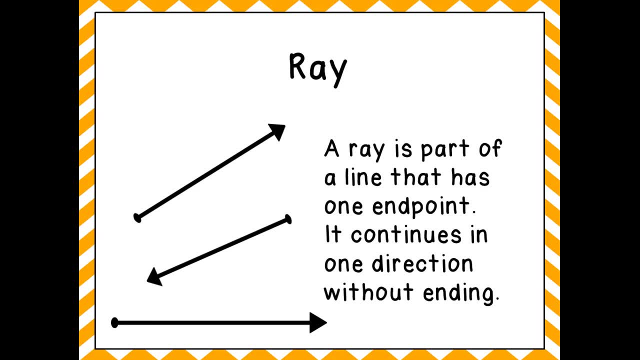 And you can tell a line segment if you see a picture, because it has two end points. on the end There are no arrows, just a lot end points or dots. Next we have a ray, And a ray is part of a line that has one end point. It continues in one direction without ending, And the way we can 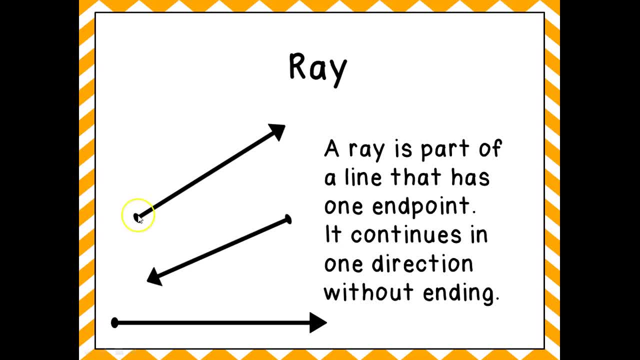 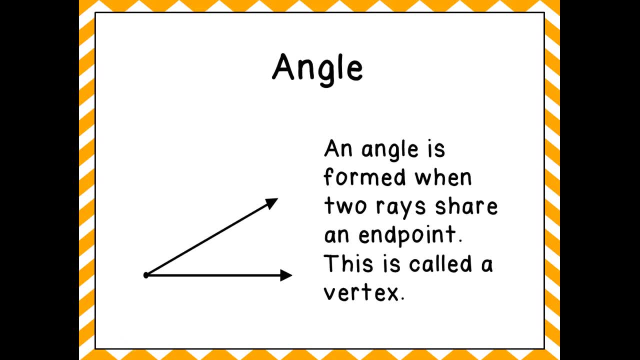 tell it's a ray is because it has an end point, has a dot on one end and an arrow telling us that it's going to continue going in that direction without stopping. The last word we want to take a look at is an angle, And an angle is formed when two rays share an end point, When the rays 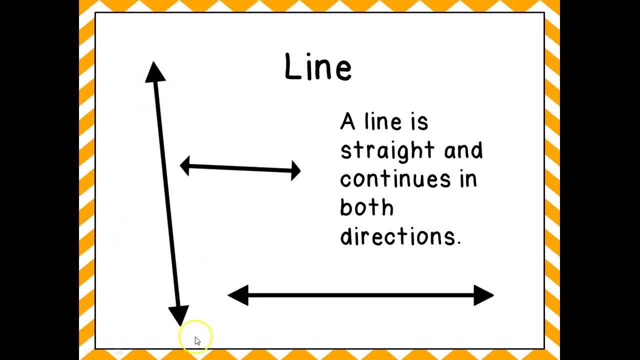 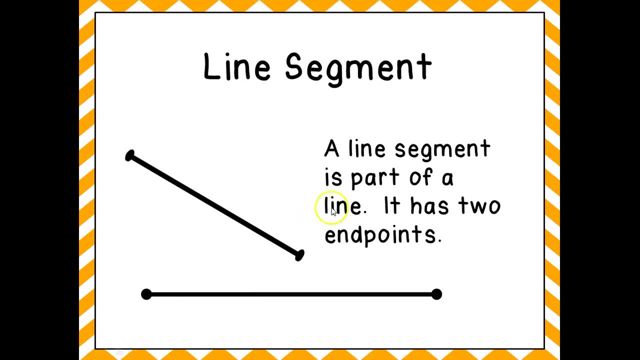 The way we can tell it's a line is because it has two arrows on either end and it's straight. Next, we have line segment, And a line segment is part of a line. So if you think about the line we just looked at, that goes on and on in both directions. a line segment is just a small piece. 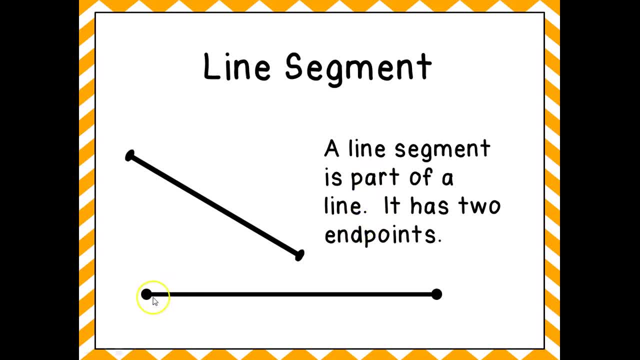 of that line And it has two end points. You see, here here's one end point. That's where it begins, And here's the second end point. Over here is where it stops. It's just a piece of that line. 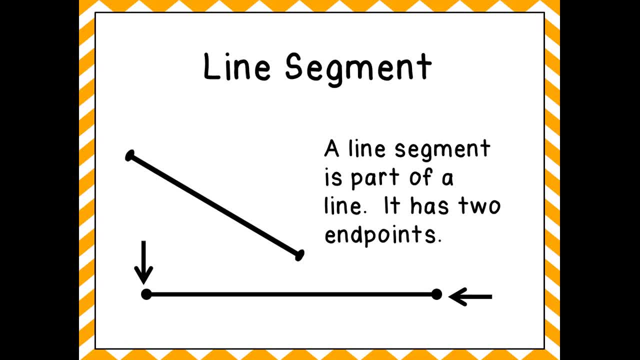 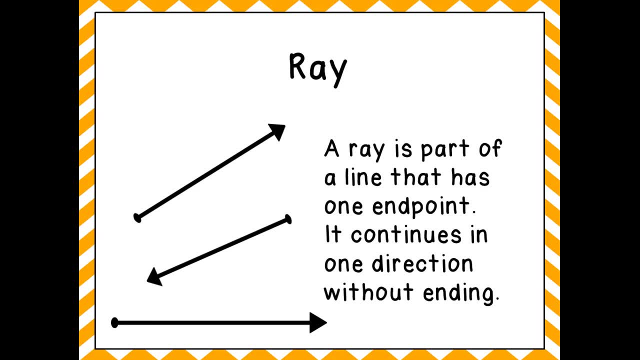 And you can tell a line segment if you see a picture, because it has two end points. on the end There are no arrows, just a lot end points or dots. Next we have a ray, And a ray is part of a line that has one end point. It continues in one direction without ending, And the way we can 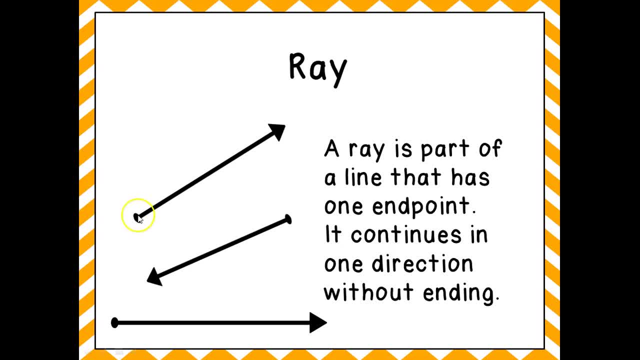 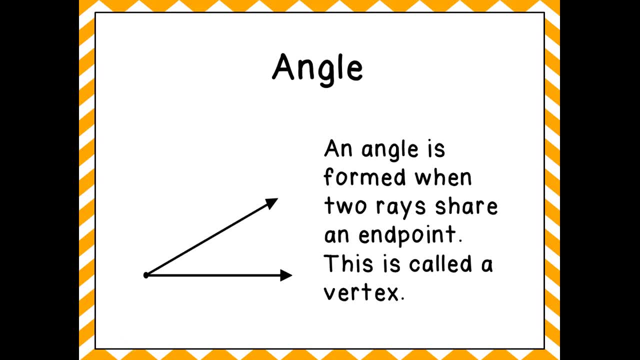 tell it's a ray is because it has an endpoint, has a dot on one end and an arrow telling us that it's going to continue going in that direction without stopping. The last word we want to take a look at is an angle, And an angle is formed when two rays share an endpoint, When 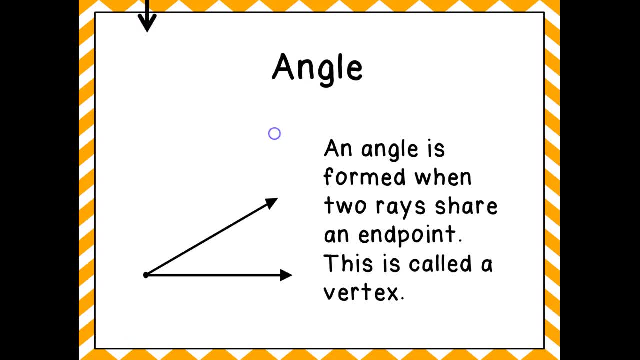 the rays are sharing an endpoint. that's called a vertex. If you take a look right there where the arrow is pointing, that would be the vertex. That would be where the two rays. you can tell it's a ray because there's a dot on one end and an arrow on the other. They're both rays, That's. 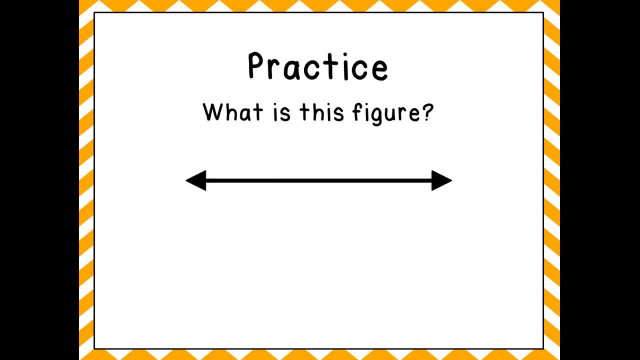 called the vertex. All right, let's do some practice. Take a look at this figure And I want you to tell me what is this figure? Is it a point, Is it a line Or is it a line segment? Take a look. 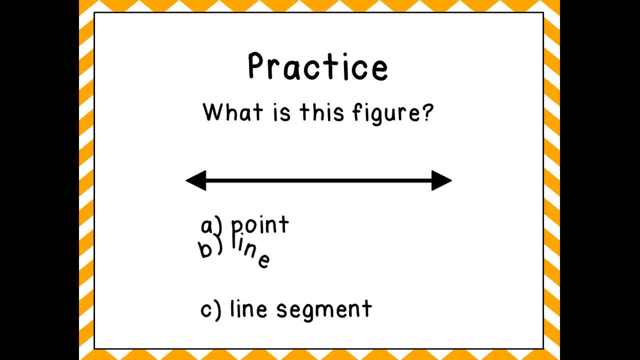 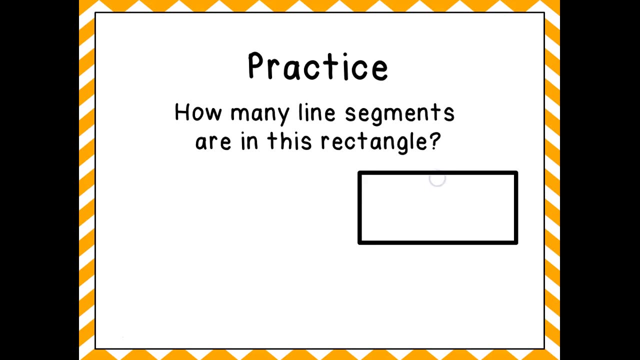 Take a moment, figure out your answer And if you chose B line, you are correct because, as you can see, it has an arrow on this side and an arrow on this side telling us that it's going to continue on in both directions. Okay, here's another practice: How many line segments are in this? 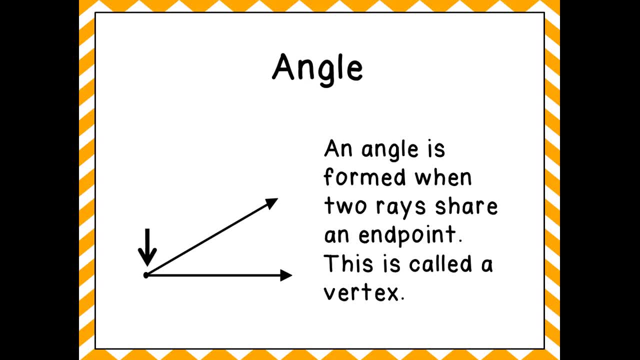 are sharing an end point that's called a vertex. If you take a look right there where the arrow is pointing, that would be the vertex. That would be where the two rays. you can tell it's a ray because it has a dot on one end and an arrow. 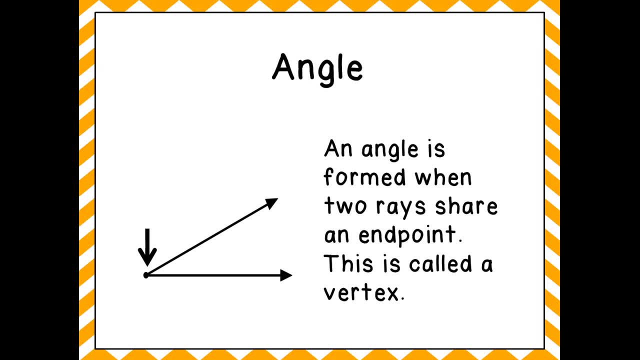 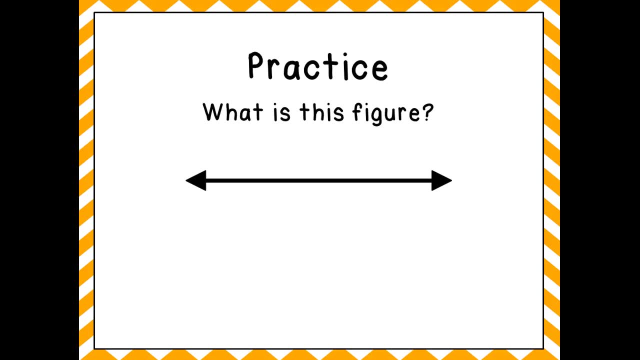 on the other. They're both rays. That's called the vertex. All right, let's do some practice. Take a look at this figure And I want you to tell me what is this figure? Is it a point, Is it a line, Or is it a line segment? Take a moment, figure out your answer. 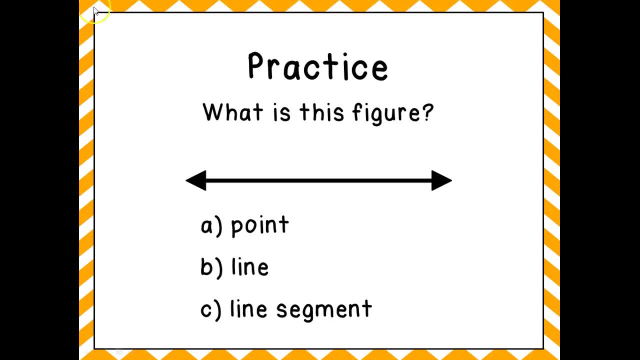 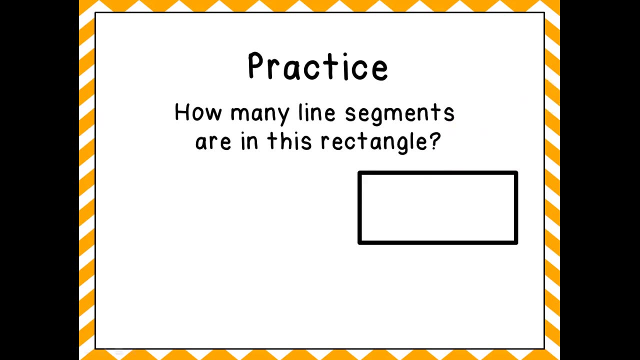 And if you chose B line, you are correct because, as you can see, it has an arrow on this side and an arrow on this side telling us that it's going to continue on in both directions. Okay, here's another practice: How many line segments are in this rectangle? Is it five, four or seven? 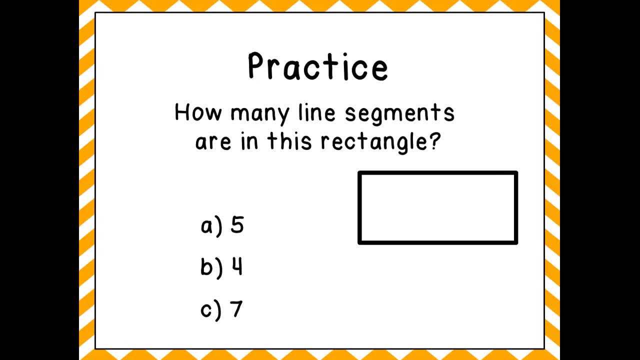 Okay, here's another practice. How many line segments are in this rectangle? Is it five, four or seven? Take a look at this figure And I want you to tell me what is this figure. Is it a line segment? 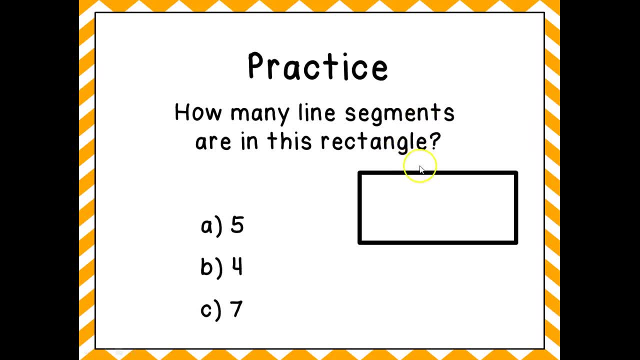 Okay, the correct answer here is letter B. There are four. Let's count them together. This is one line segment. Here's your end point. another end point, Here's your second line segment, your third one right here and number four right over here. 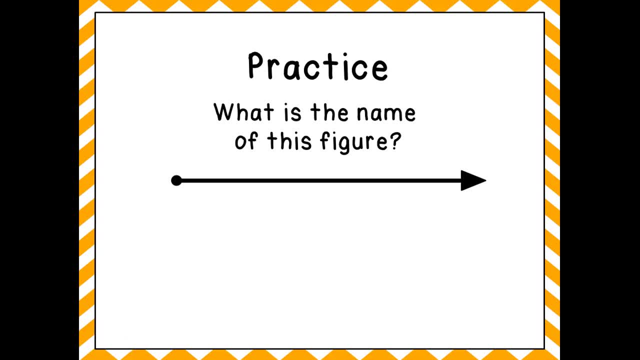 Okay, here's another one. What is the name of this figure? Is this figure a line, Is it a ray or is it a line segment? Go ahead and choose your answer. Okay, if you chose B ray, you are correct. You can see here. it has an end point on this end, and. 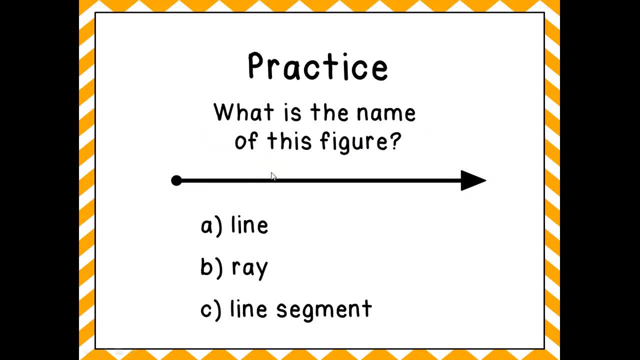 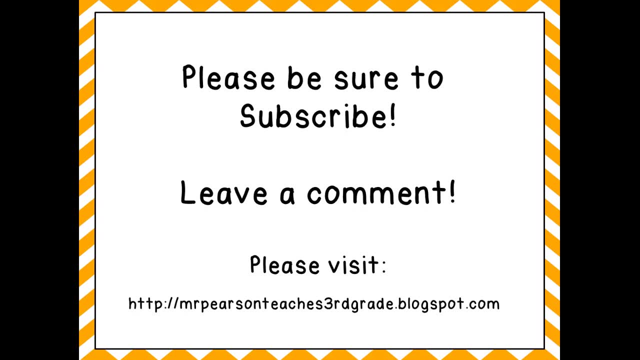 an arrow on this end. It's telling me that it continues on in just one direction. Alright, please be sure to subscribe to the channel below. Click the subscribe button below so you can keep updated with what we've got going on. Also, if you.